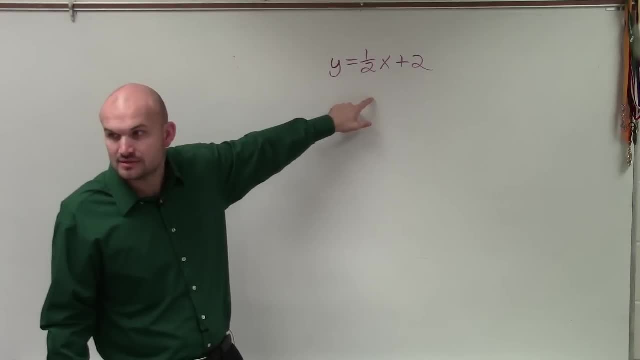 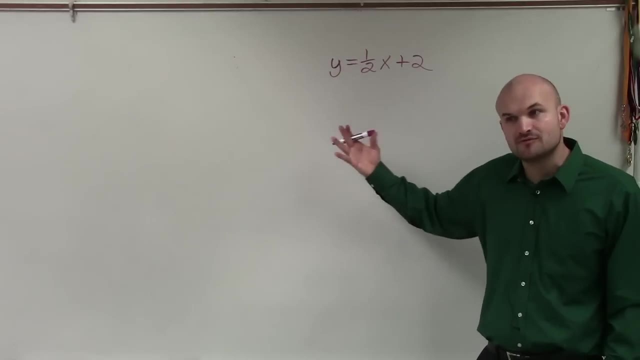 on graphing, I can always use a table of values Correct. So when I give you a problem like this on your test, I don't ever want to see something blank because there's no reason for it. You guys should all know you can always go back to doing that work. Determine x values. 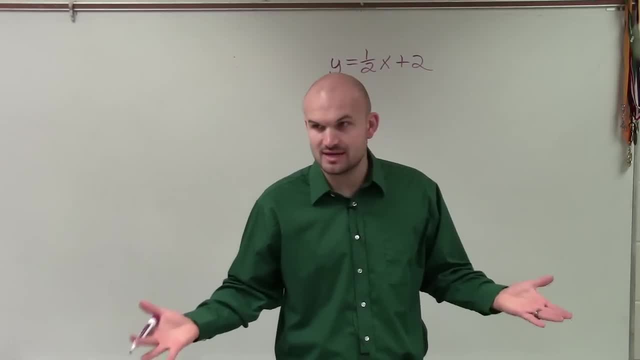 plug them in and find the y value Right. Does everybody understand that? Yes, So even if you have trouble with what I'm about to go over, still you can always go back to using table of values. So I don't want to see any blank. 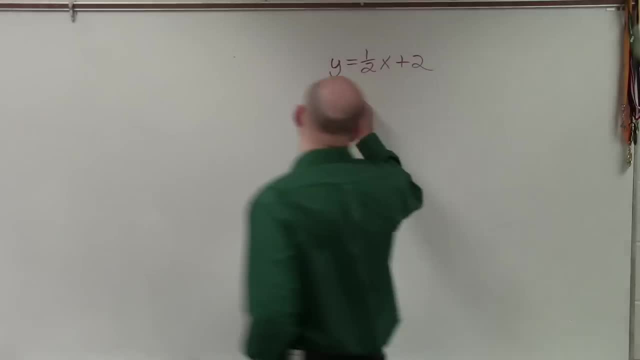 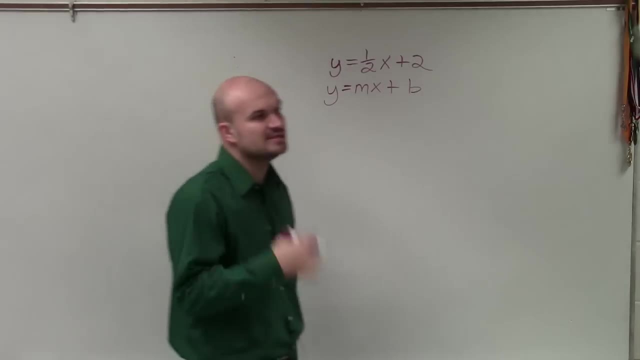 graphs when we go through to take the test Now. last class period, which I will walk around and check your work, we talked about writing equations in slope-intercept form, And the reason why that was kind of so important is because, rather than using a table of values, 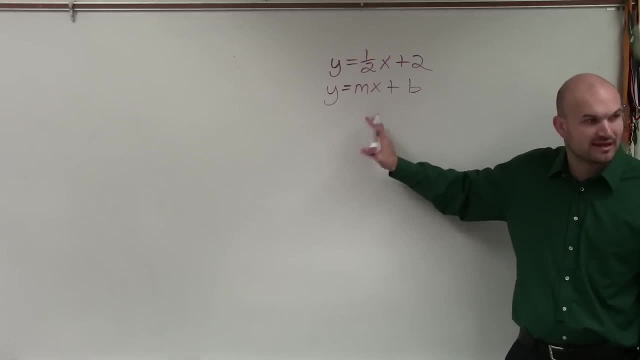 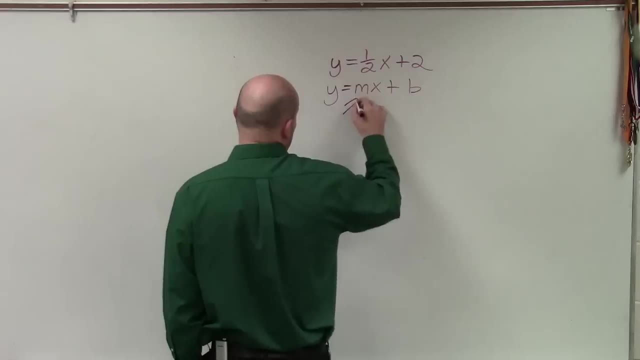 which you can do. it's much easier to use slope-intercept method when graphing an equation. when it's in slope-intercept form, It's much easier to use this method. And basically, what I spoke about last class period was this: m represents your slope and b represents 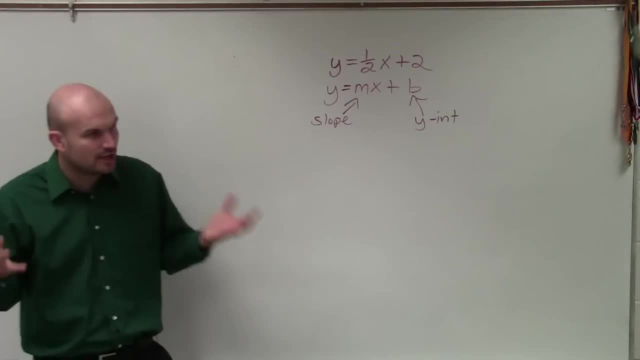 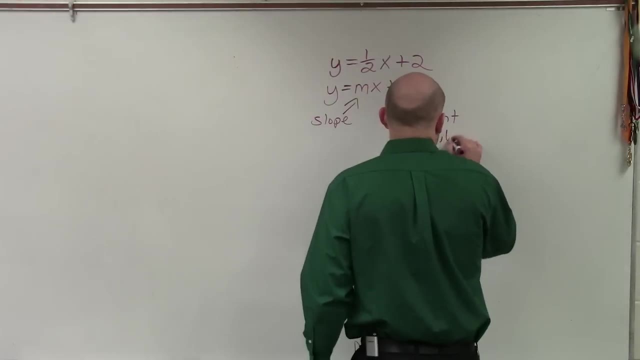 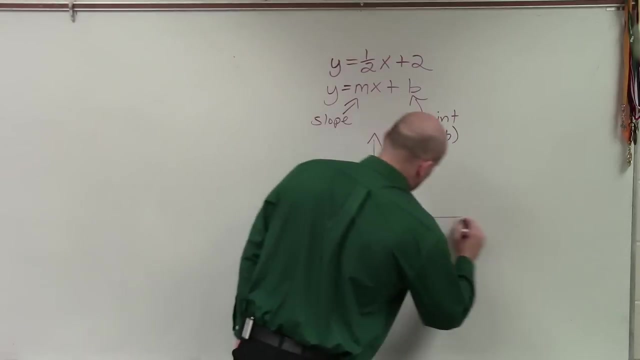 your y-intercept And to graph them. it's very important that we understand the difference between intercept and slope. Y-intercept is the point where the graph crosses the y-axis. It is a coordinate point, a point on the graph where it's going to cross the y-axis And 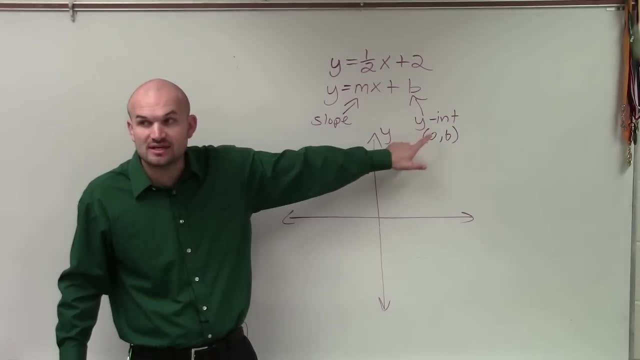 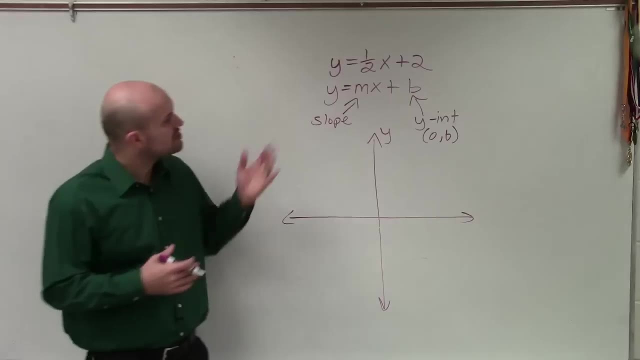 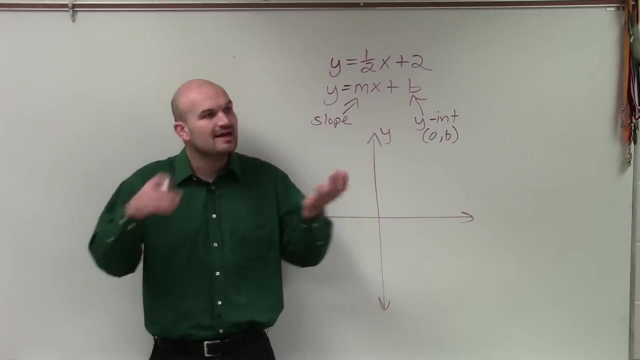 so you can see I write it as a coordinate point. The x value is always equal to the y-intercept And b is always going to be your y-value. The slope is not a point, The slope is the ratio. Remember, ratio is comparison. It's a comparison. It's the comparison of. 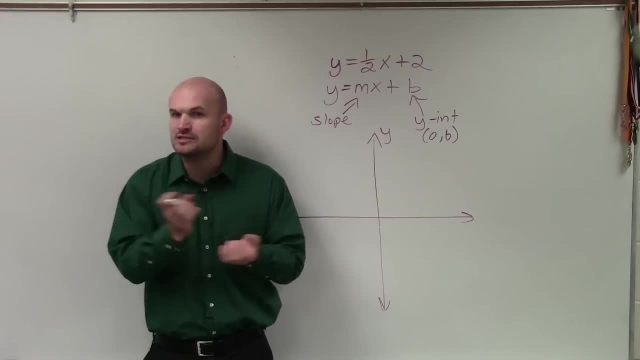 the change in y-values over the change in x-values between any two points. So we always like to write slope as a fraction And you guys can think of it as rise over run. I'm not really too fond of the word. I'm not really too fond of the word. I'm not really. 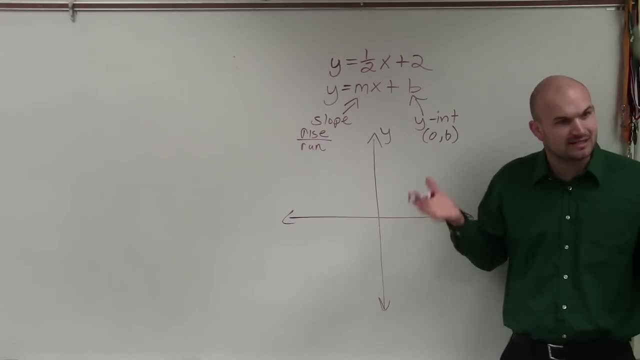 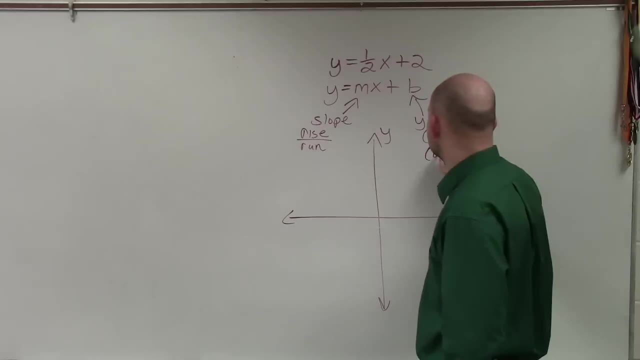 too fond of the word rise over run, But basically you just want to think of it, though, as a fraction. Always write your slope as a fraction, So in this case my y-intercept is 0, 2.. So 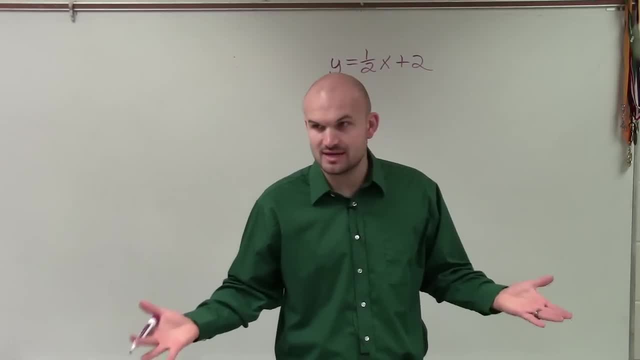 plug them in and find the y value Right. Does everybody understand that? Yes, So even if you have trouble with what I'm about to go over, still you can always go back to using table of values. So I don't want to see any blank. 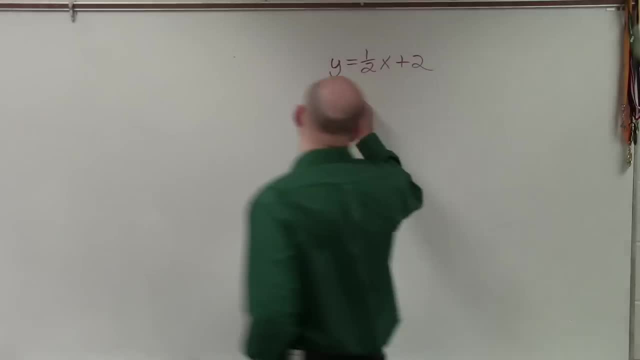 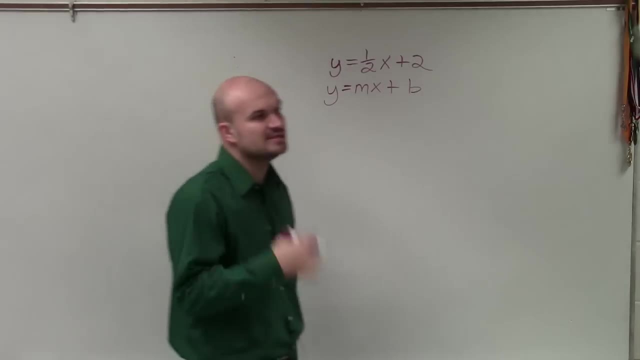 graphs when we go through to take the test Now. last class period, which I will walk around and check your work, we talked about writing equations in slope-intercept form, And the reason why that was kind of so important is because, rather than using a table of values, 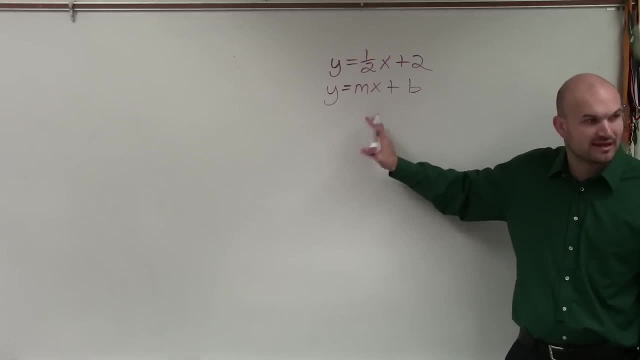 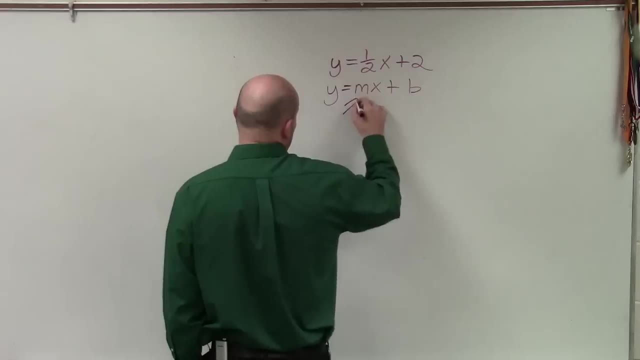 which you can do. it's much easier to use slope-intercept method when graphing an equation. when it's in slope-intercept form, It's much easier to use this method. And basically, what I spoke about last class period was this: m represents your slope and b represents 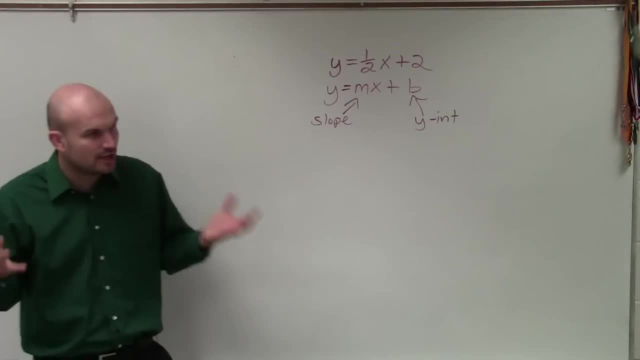 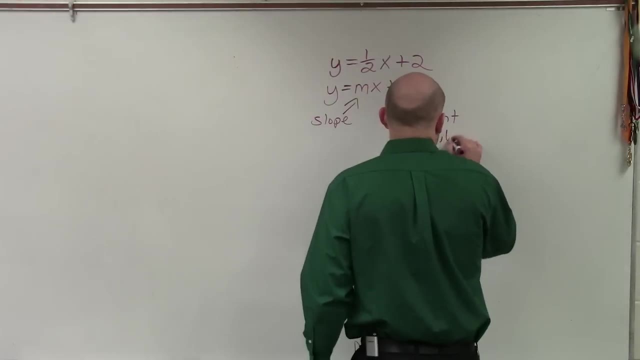 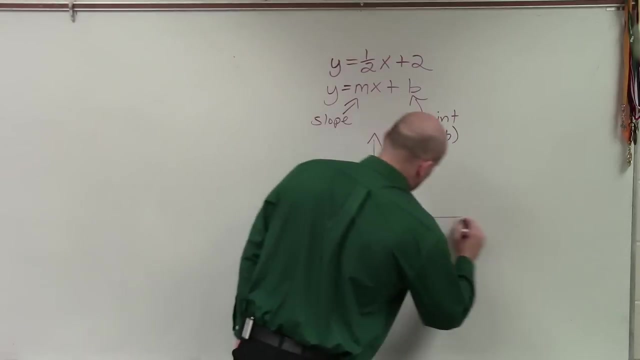 your y-intercept And to graph them. it's very important that we understand the difference between intercept and slope. Y-intercept is the point where the graph crosses the y-axis. It is a coordinate point, a point on the graph where it's going to cross the y-axis And 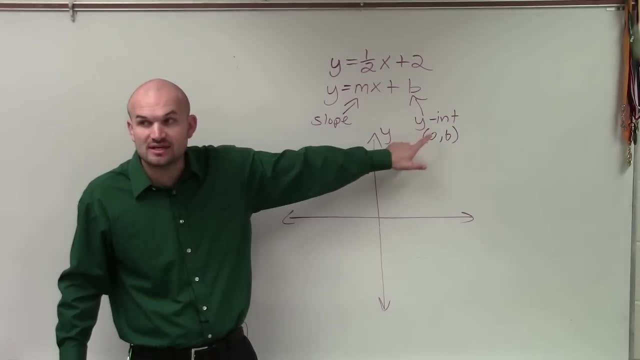 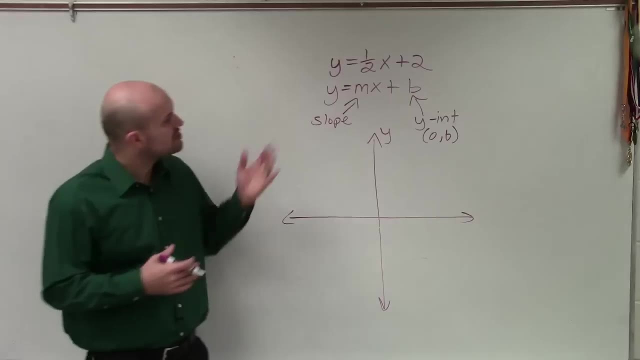 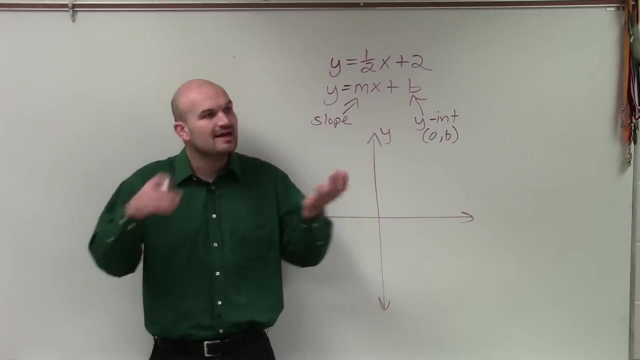 so you can see I write it as a coordinate point. The x value is always equal to the y-intercept And b is always going to be your y-value. The slope is not a point, The slope is the ratio. Remember, ratio is comparison. It's a comparison. It's the comparison of. 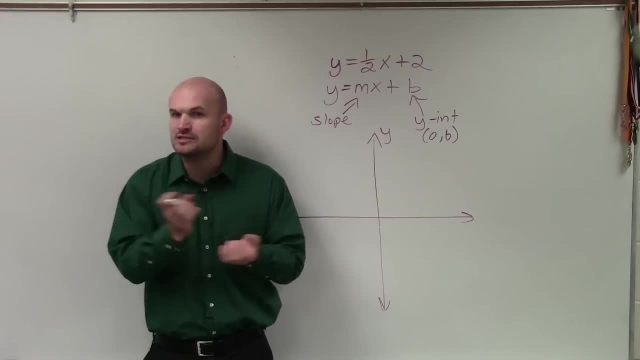 the change in y-values over the change in x-values between any two points. So we always like to write slope as a fraction And you guys can think of it as rise over run. I'm not really too fond of the word. I'm not really too fond of the word. I'm not really. 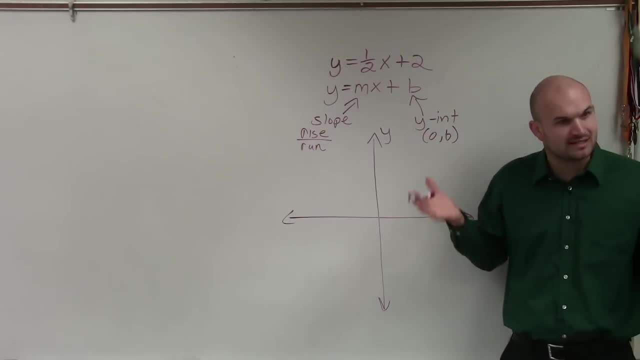 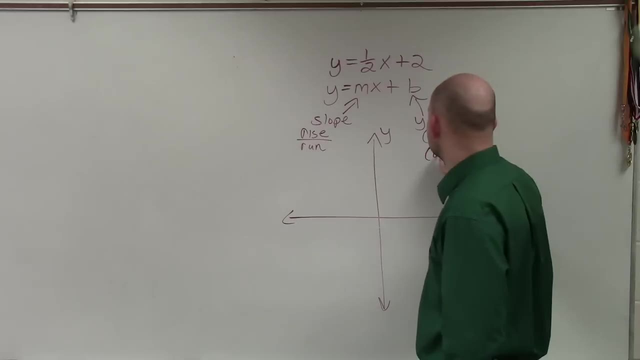 too fond of the word rise over run, But basically you just want to think of it, though, as a fraction. Always write your slope as a fraction, So in this case my y-intercept is 0, 2.. So 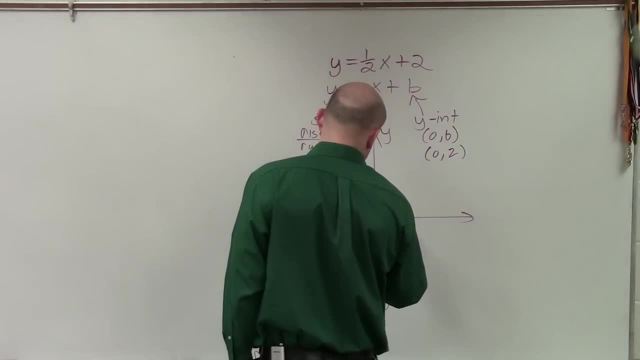 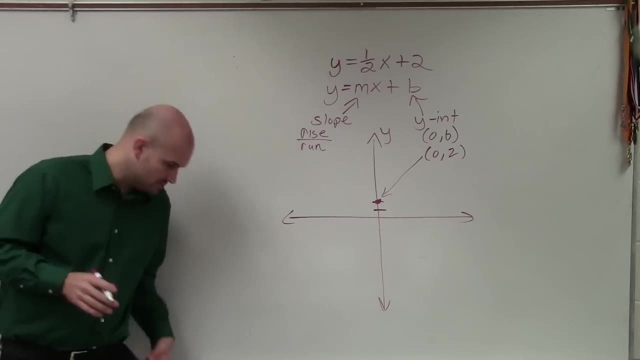 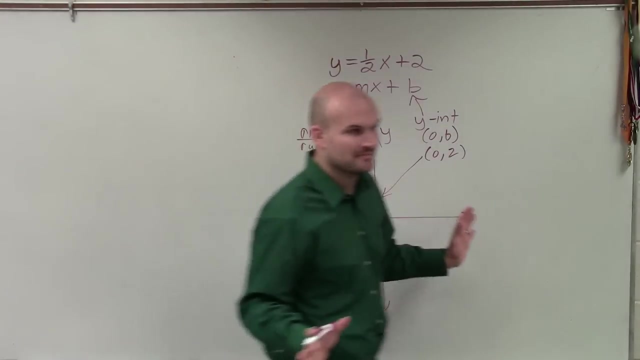 I can plot 0, 2.. Make that nice point right there. Does everybody follow me? Is everybody with me? I just plotted the y-intercept. Everybody should hopefully go with the y-intercept Now. the next thing is my slope, which is: 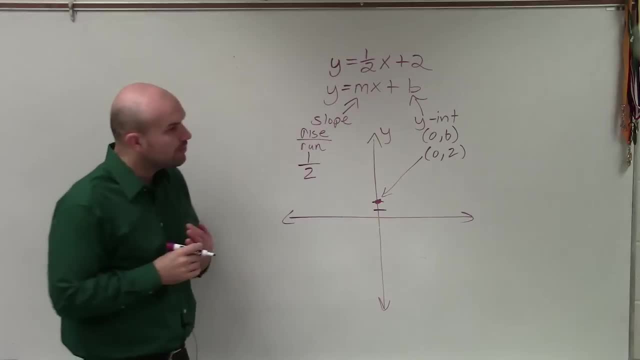 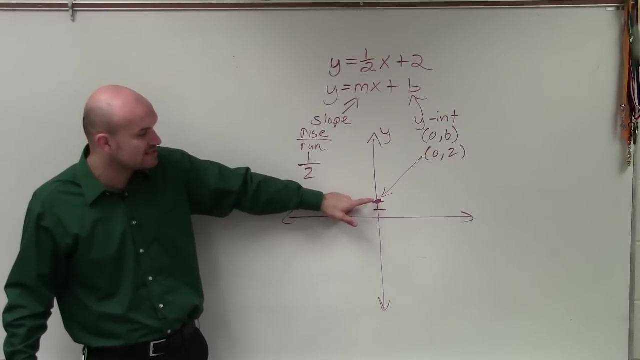 my rise over 1, my 1 over 2.. So what that states is the change between any two points. the change in the y-values between any two points is positive 1.. So if I have one point to graph a line, I need two points. That means that the change between any two points, the 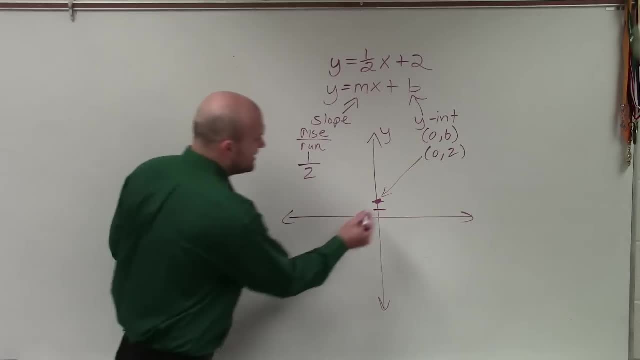 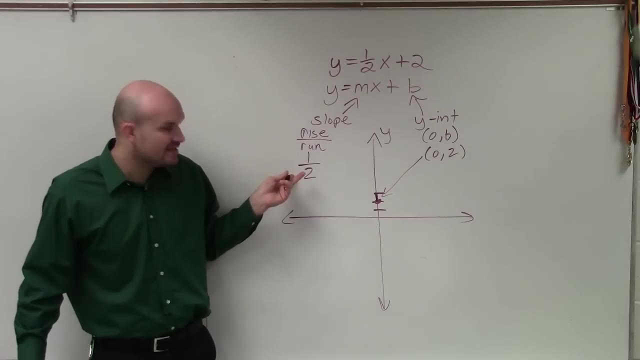 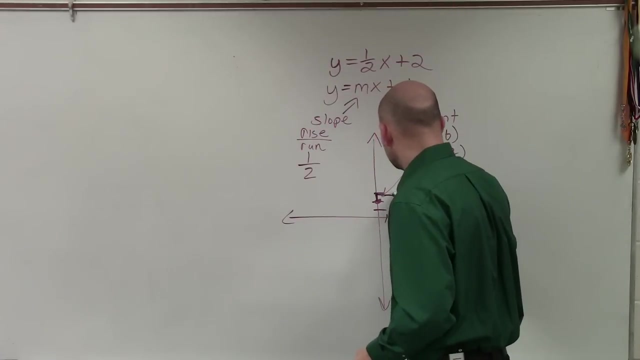 y-values is positive. 1. To find the next point, I need to go up one. Then the change in the x-values is positive. 2. So to find the next point, I need to go to the right two. And when you do that, when you follow those steps, you create what we. 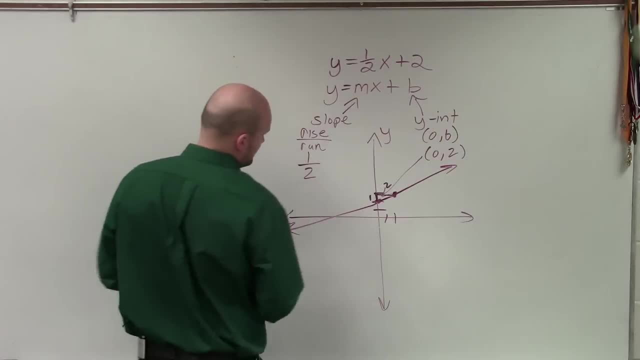 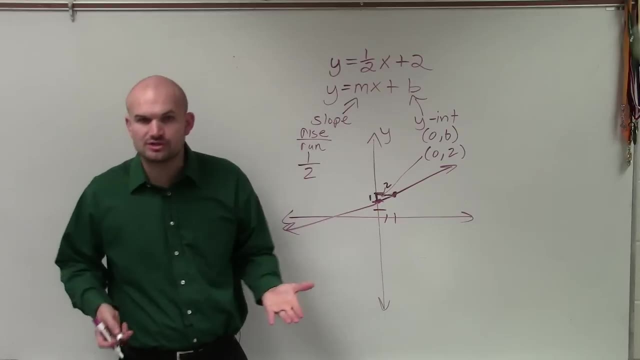 call a slope triangle And, ladies and gentlemen, all we need is two points to graph And that's it, Boom Done. You don't need to do six points, like you guys did with your functions. You can do that, but you don't have to. We just need two points And you can just continue. 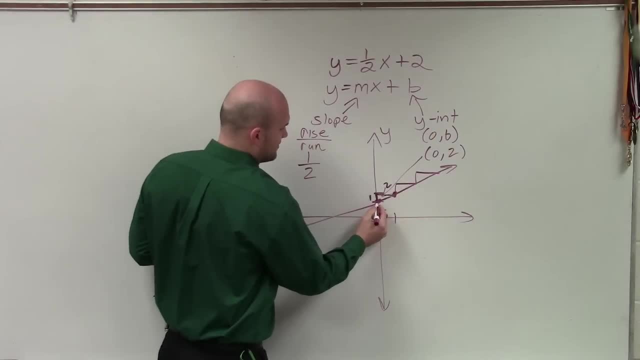 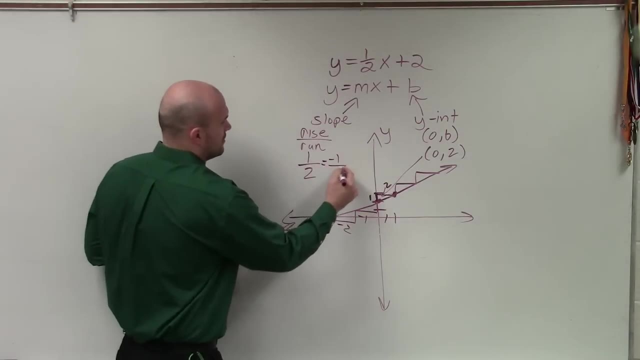 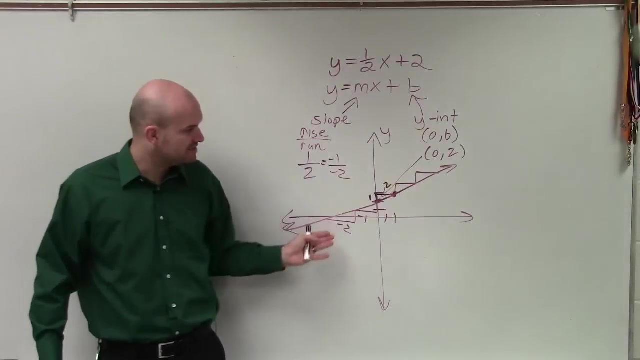 If you guys notice, the slope is the same. You could also do negative 1, negative 2, because negative 1 over negative 2 is going to give you the same points. So do you guys see how that slope is, that constant ratio, that constant comparison between any two points? 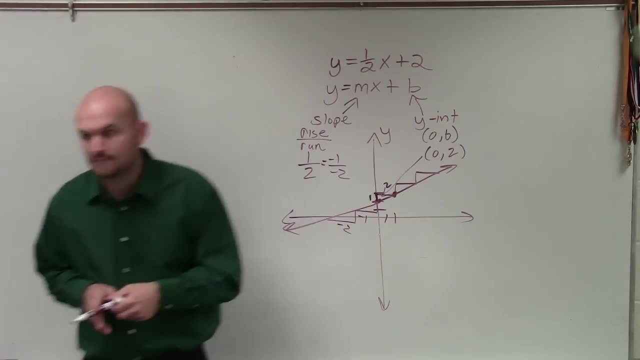 But to graph this, all you need is those two points. OK, Good, Yes, OK, Let's go over one more, then I'll give you. 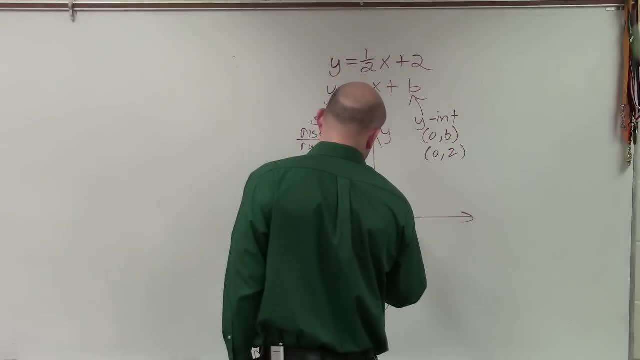 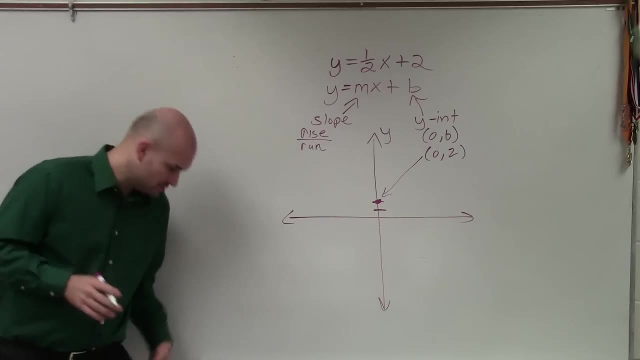 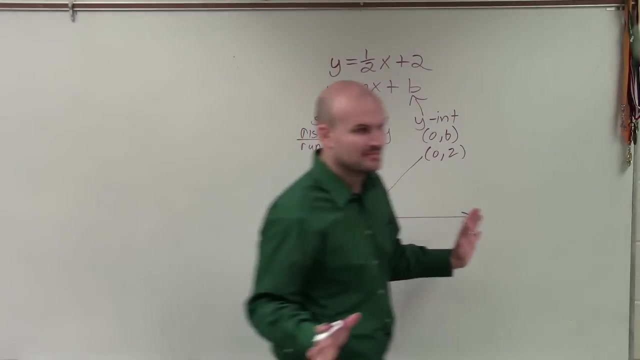 I can plot 0, 2.. Make that nice point right there. Does everybody follow me? Is everybody with me? I just plotted the y-intercept. Everybody should hopefully go with the y-intercept Now. the next thing is my slope, which is: 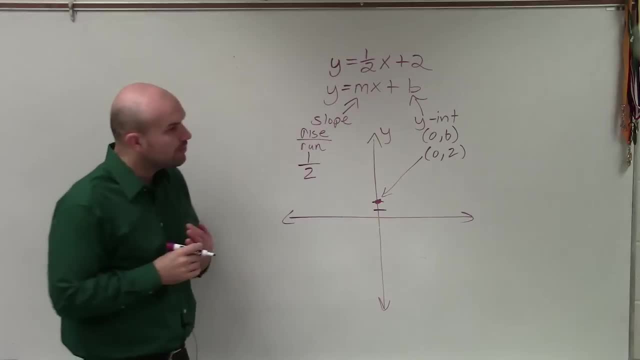 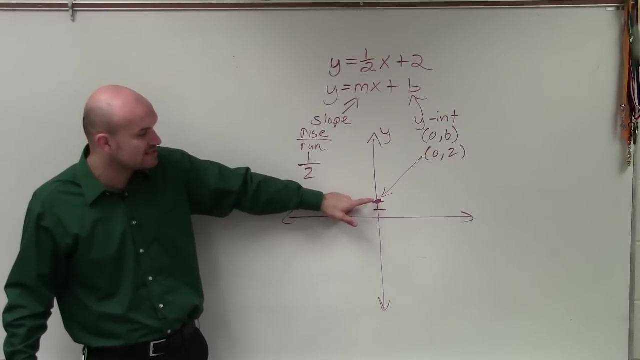 my rise over 1, my 1 over 2.. So what that states is the change between any two points. the change in the y-values between any two points is positive 1.. So if I have one point to graph a line, I need two points. That means that the change between any two points, the 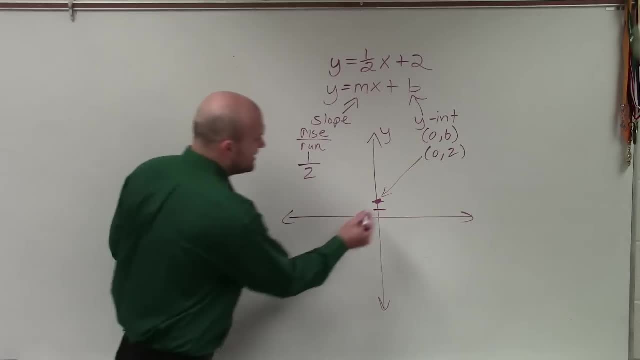 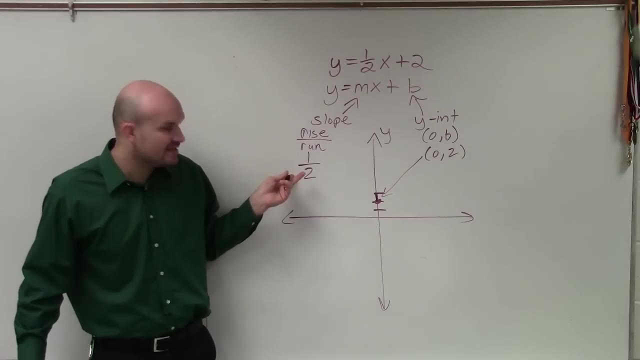 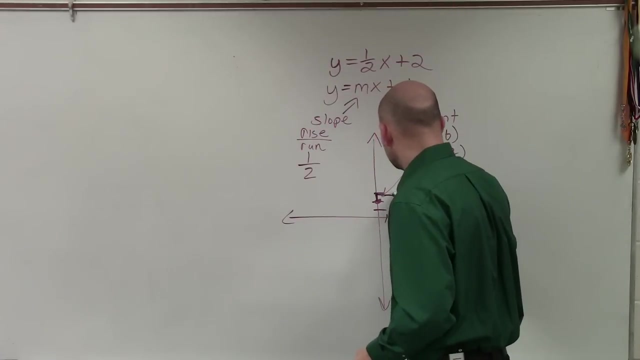 y-values is positive. 1. To find the next point, I need to go up one. Then the change in the x-values is positive. 2. So to find the next point, I need to go to the right two. And when you do that, when you follow those steps, you create what we. 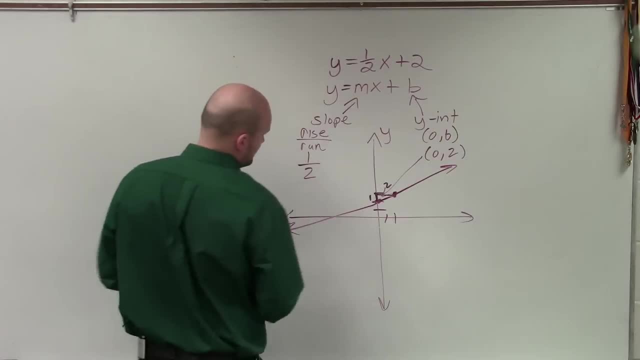 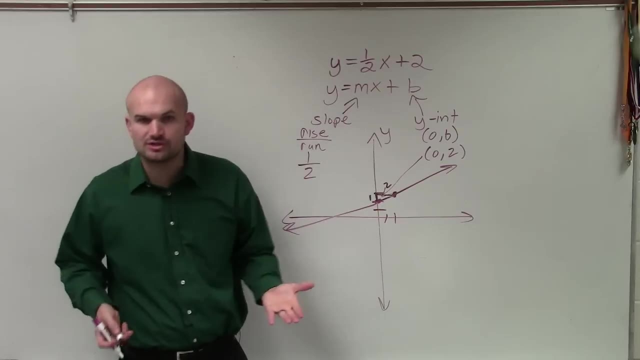 call a slope triangle And, ladies and gentlemen, all we need is two points to graph And that's it, Boom Done. You don't need to do six points, like you guys did with your functions. You can do that, but you don't have to. We just need two points And you can just continue. 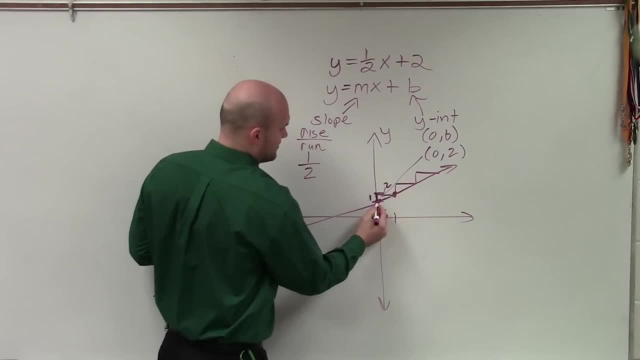 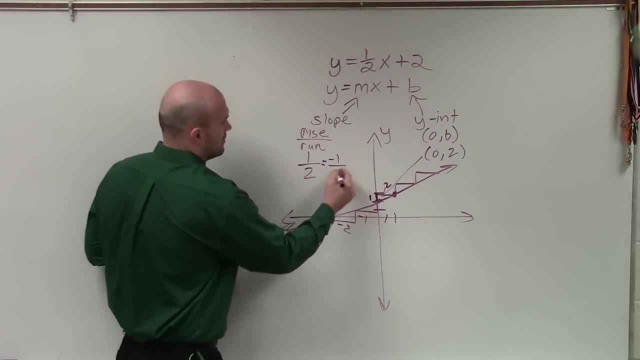 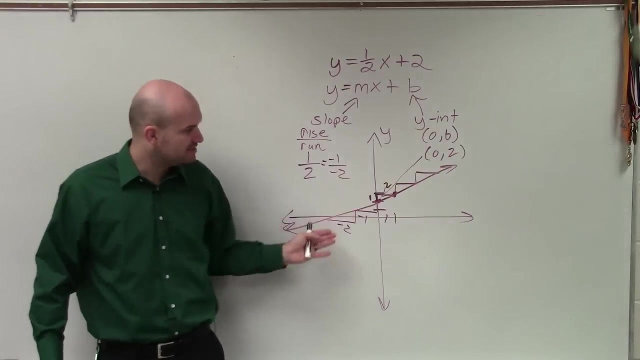 If you guys notice, the slope is the same. You could also do negative 1, negative 2, because negative 1 over negative 2 is going to give you the same points. So do you guys see how that slope is, that constant ratio, that constant comparison between any two points?